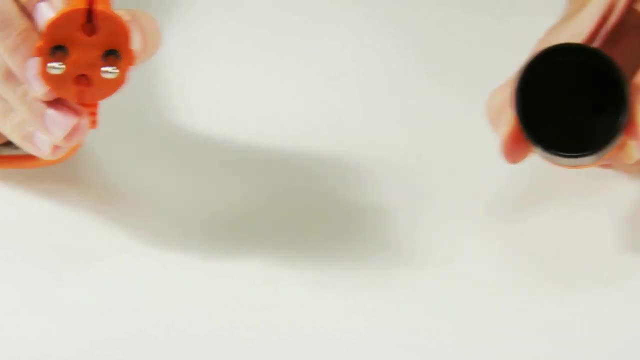 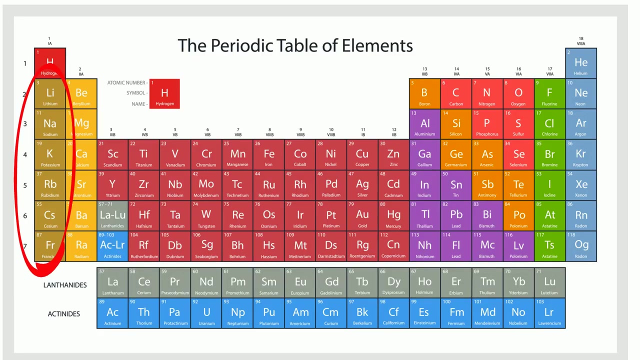 Metals are good conductors of heat and electricity. All but mercury are solid at room temperature. The alkali metals are group 1 and they're the most reactive of all metals. They don't occur in nature in their element form, but are always found in a compound. 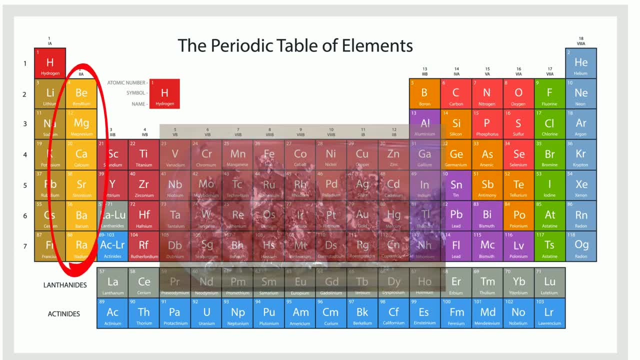 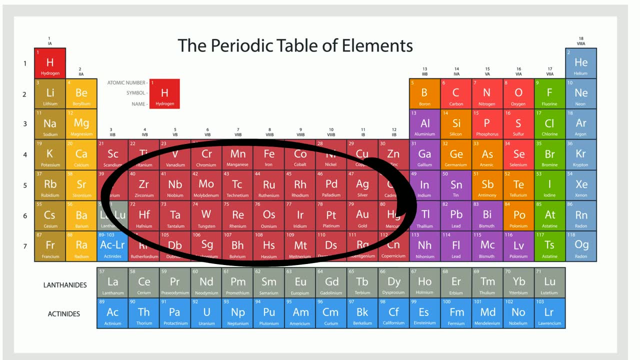 The alkaline earth metals- group 2, are shiny, ductile and malleable and they combine with other elements. The transition metals, groups 3 through 12, are most familiar metals because they often occur in nature uncombined. The lanthanide series, elements 51 through 71, are found at the bottom. 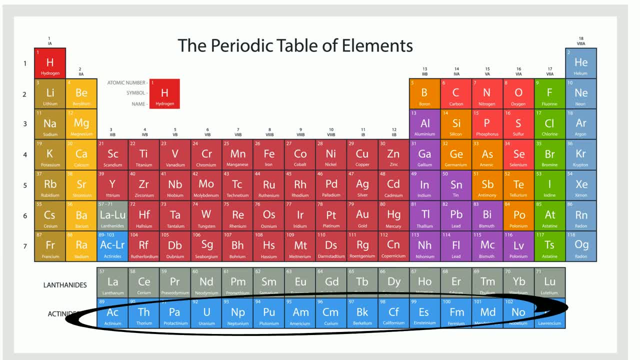 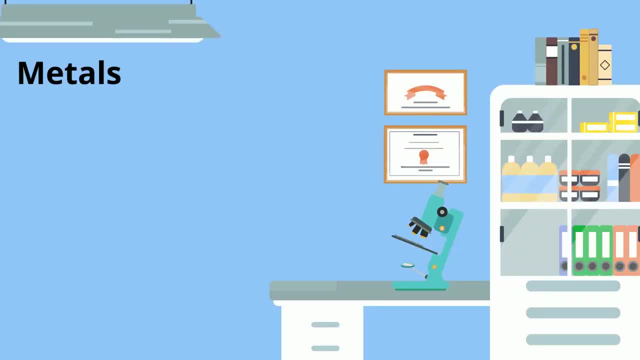 of the periodic table and the actinine series are elements 89 through 103.. If you were to summarize the properties of the metals- shiny conductors, malleable, ductile and metal- you'd know that the nonmetals are the opposite: They're dull. 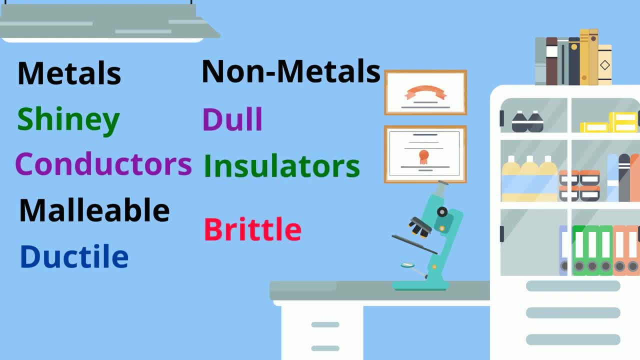 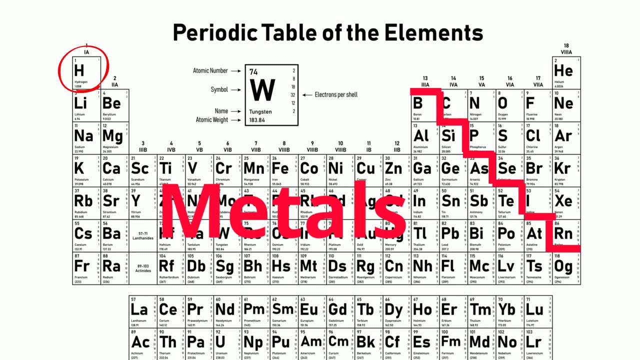 insulators and brittle Nonmetals are elements that are usually gasses or brittle solids at room temperature. Most can form ionic and covalent compounds and are located to the right of the zigzag staircase. The halogens, which are group 17,, are the most reactive of the nonmetals. These elements combine. 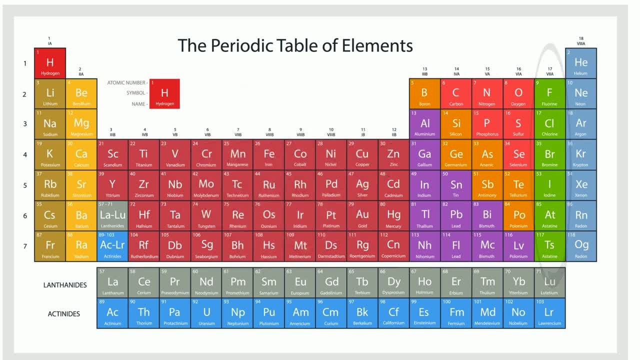 combine with group 1 to form salts. The noble gases- group 18, exist as isolated atoms. They are all stable because their outer energy level is full. Hydrogen, which is the only non-metal located to the left of the zig-zag staircase, is located at the top of group. 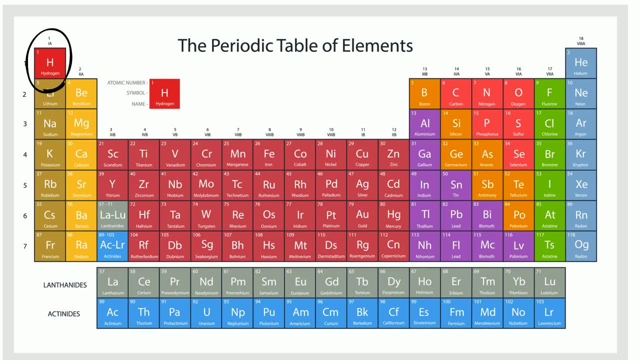 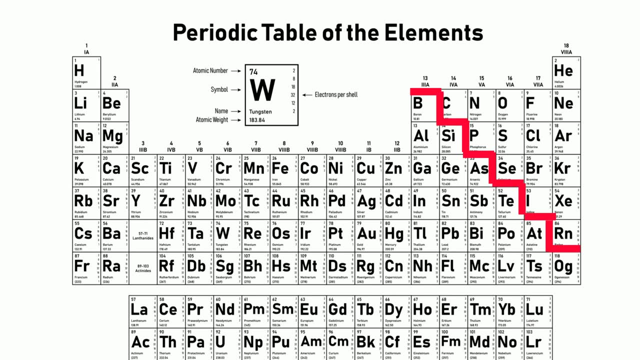 1 because of reactivity, and it only has one valence, electron. The metalloids are part of the mixed groups, groups 3-17, and they can be metals, non-metals and metalloids. One side of the metalloids actually touch the zig-zag staircase. Be careful with aluminum. 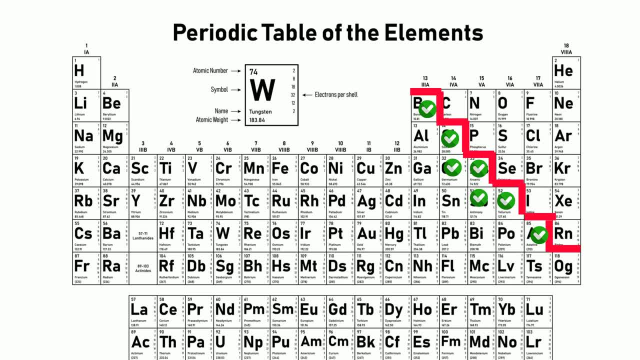 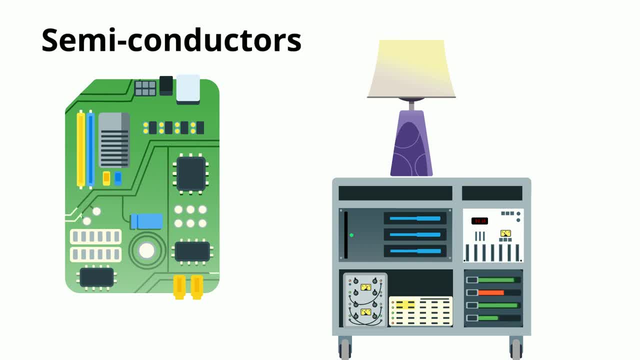 though They have qualities of metals and non-metals. They are also known as semi-conductors. They are widely used in technology. For example, silicon is used in computer chips and germanium is used in lights and lamps. If you'd like to know more about the periodic table, this playlist will help.